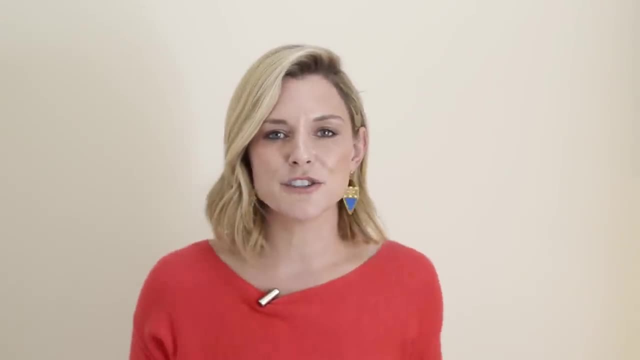 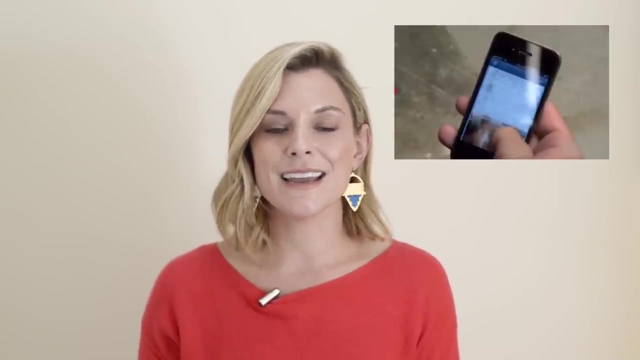 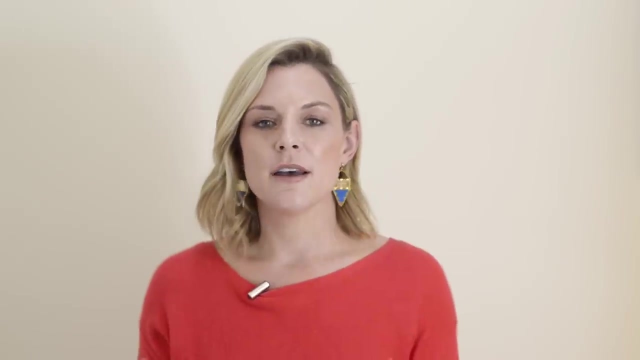 story, And on and on, and on, and the speaker can be one or two minutes in and they haven't said anything interesting. Guess what? Now your audience is on their phone. We can do better you. My name is Ann Ricketts. I'm the founder of Lighthouse Communications And for a living I help people deliver more effective. 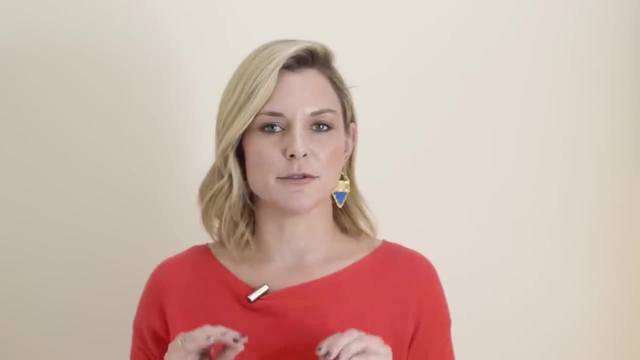 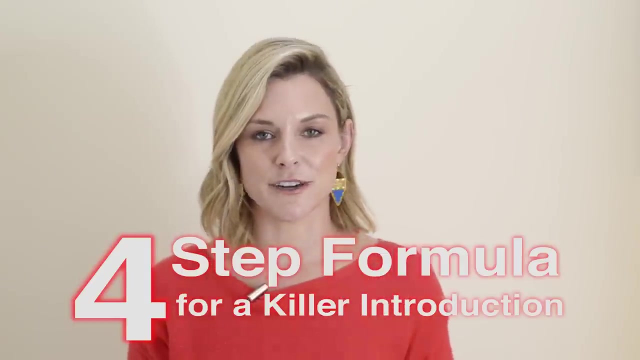 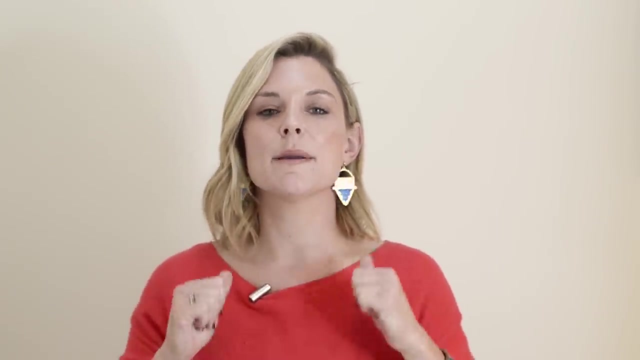 presentations. I strongly believe that introduction is the most crucial piece to your presentation And in this video, I'm going to share with you a four-step formula for a killer introduction. And if you follow this, not only will your audience be leaning in wanting to hear more, but you will be. 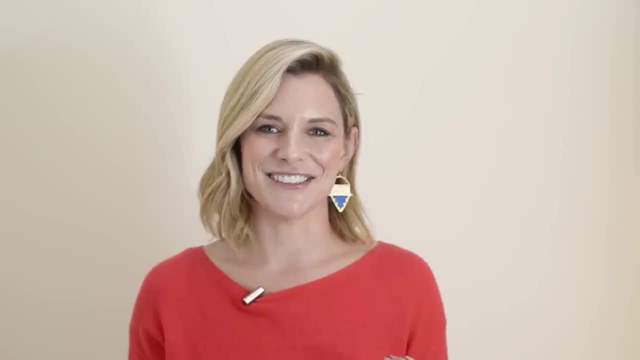 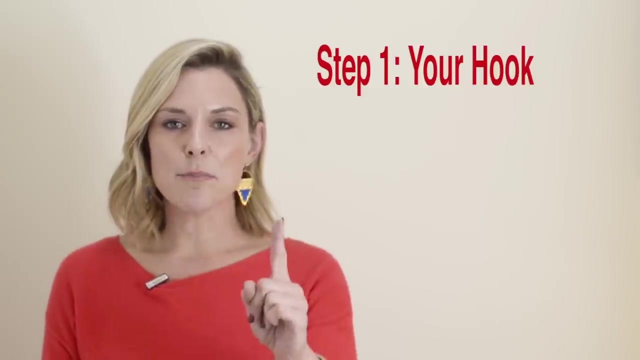 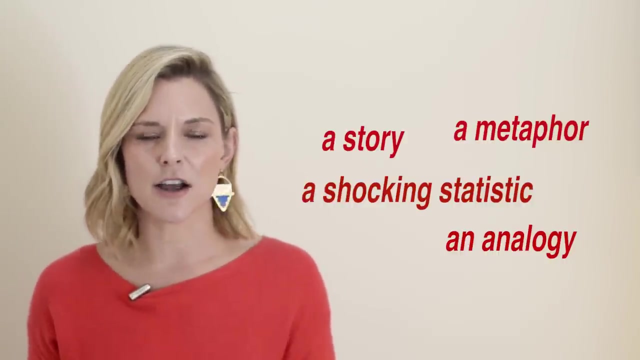 bursting at the seams with confidence from giving such an amazing introduction. You ready for this, Ready for the formula? Step one is your hook: A story, an analogy, a metaphor, a shocking statistic, a question or a combination of those things, Something interesting and vivid. 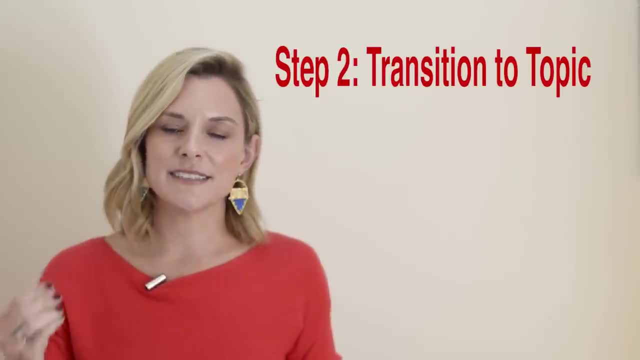 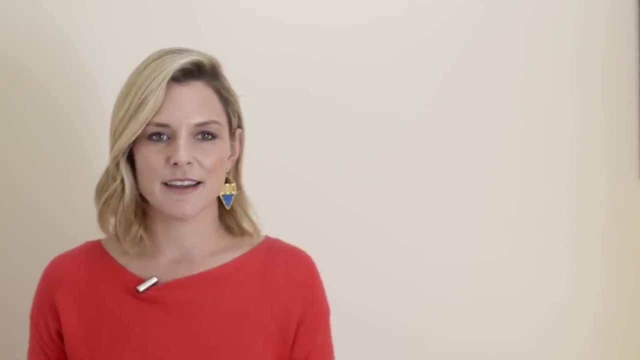 right away to pull them in. Step two is the transition to your topic Bridge, the gap between that hook and what you're going to talk about today. You can say something like You might be wondering what CSI knows has to do with presentations. I tell that story because this story illustrates. 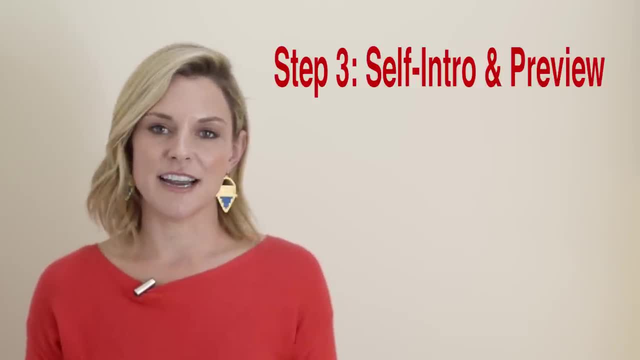 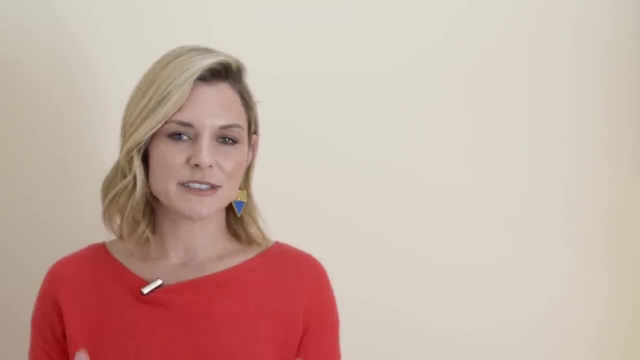 Step three is your self-introduction and a preview of your of your talk. If you don't know the audience yet, you can briefly introduce yourself. Just give them the most interesting things from your background that directly relate to your topic. And remember you can establish credibility throughout your. 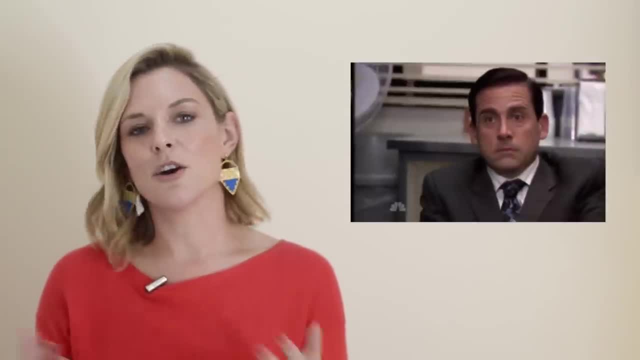 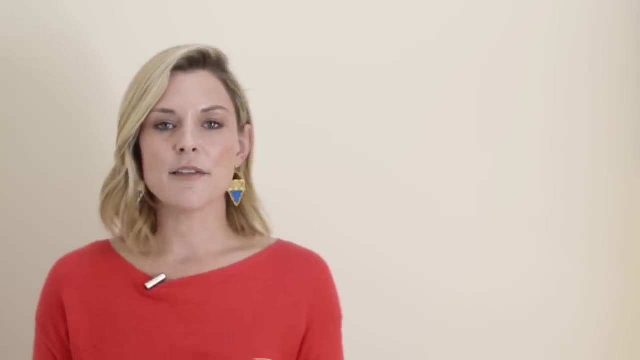 talk, so you don't have to give them a full bio And then go ahead and preview what are the goals of your talk. what will you be covering? Step four is the benefit for your audience. Tell the audience what they will gain from listening to your talk. Don't assume that they already know. You should be specific. 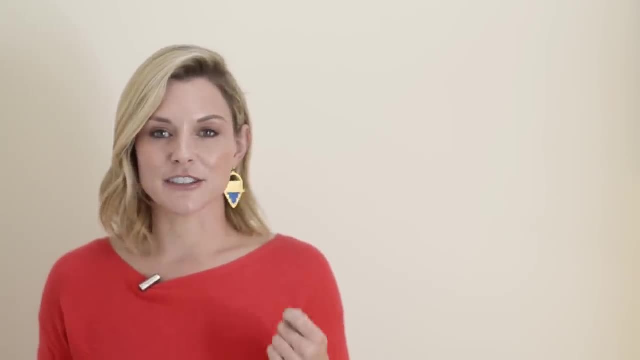 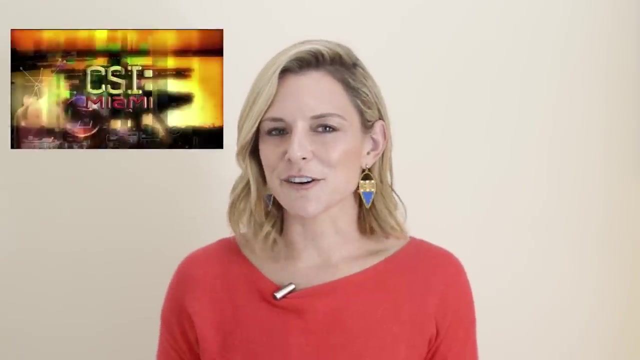 Now that you know the four steps for giving a killer introduction, let's break it down and let's look at the introduction to this video. Have you ever seen Law and Order or CSI? Well, if you have, you know how those shows start. They.